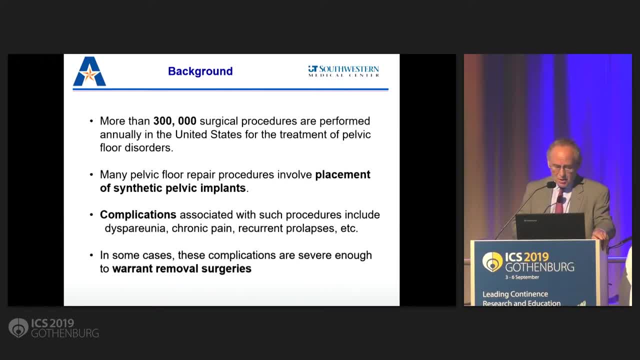 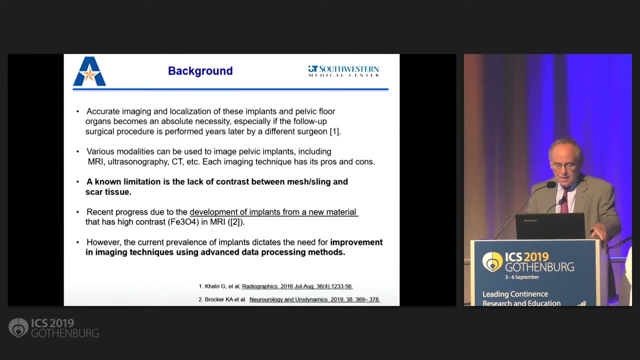 that we have lots of surgeries in the field and many of them need mesh and we see complications and we are struggling to remove these, and it's especially true in my place, tertiary care center in Dallas. We have a lot of technologies available. The imaging technology is already. 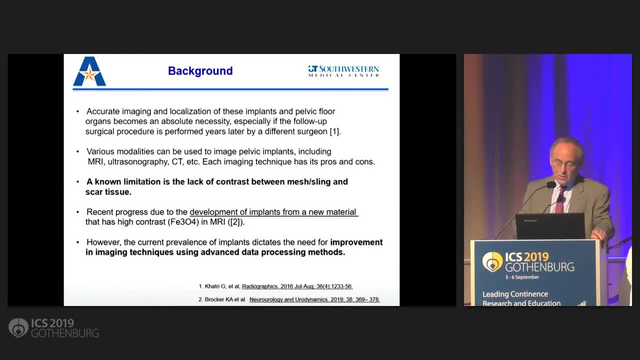 available, but the problem is to define where the mesh is or where the sling is at times in scar tissues, and there has been some work done by John Delancey and his group to try to basically render these implants visible and we're looking at a different way to look. 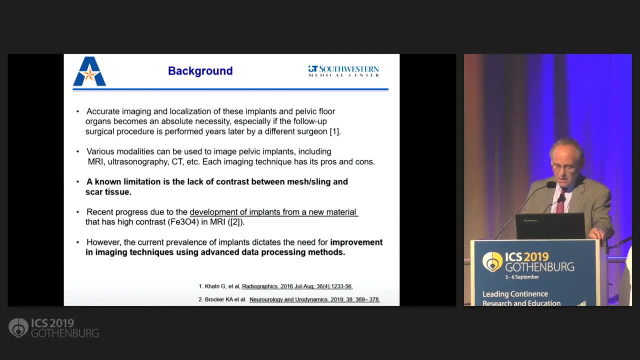 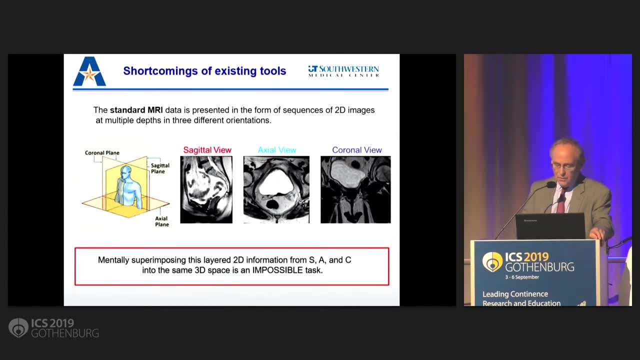 at that, which is improving our imaging technology and using advanced data processing methods to do that. So here is the example of what we're struggling with. This is an MRI with three different views- sagittal, axial and coronal- and putting 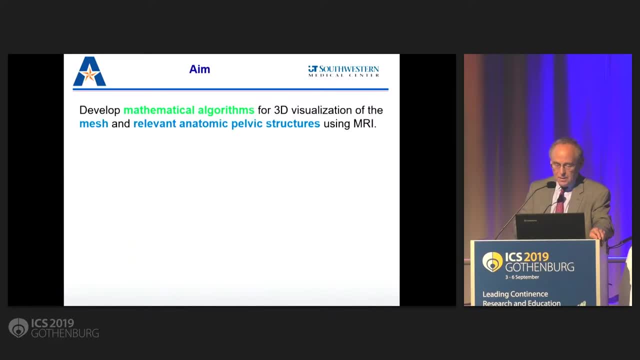 them together in three dimensions is really impossible- at least I can't. So the help of the mathematicians is to develop algorithms for us to be able to sort out where is the mesh and where are the relevant anatomic pelvic structures. If you take the slices: 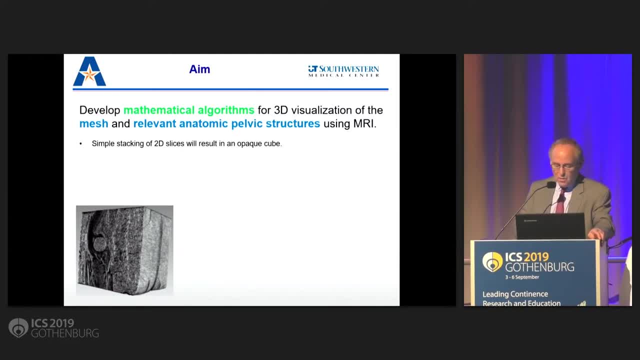 of an MRI and put them together, you get a big opaque cube. that doesn't work. If you do transparency technologies, you withdraw images to see the key things. that doesn't work either. you're missing important features. The best technology is the MRI. 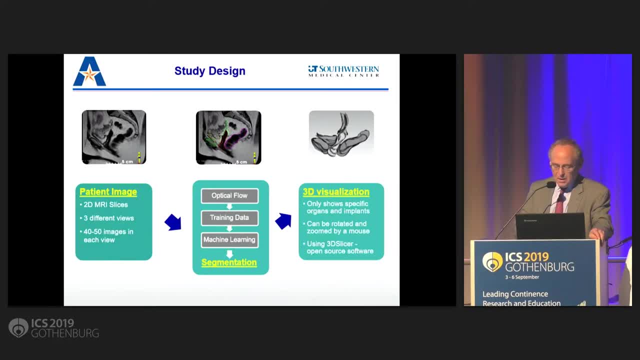 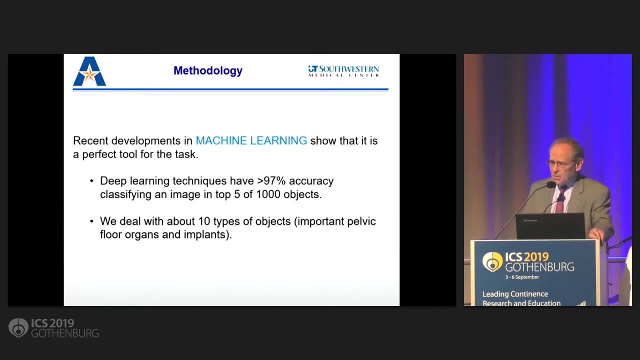 The technology they're offering right now is called image segmentation, and this is based on basically this follow-up process here going from optical flow to training the machine and then to bring that into a 3D slicer. So the machine learning can in fact recognize objects quite readily. They have a very high 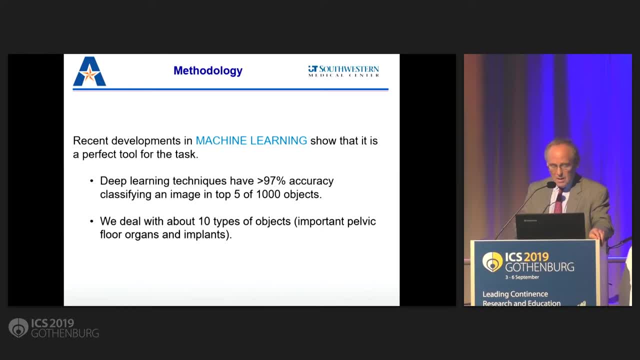 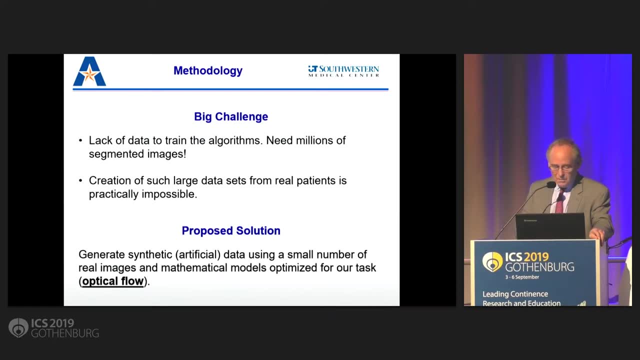 accuracy for a large number of objects. so picking up about 10 pelvic structures should be very doable for that technology. at present The problem is that you have to train the system, meaning thousands of images, and we don't have them because we don't have thousands. 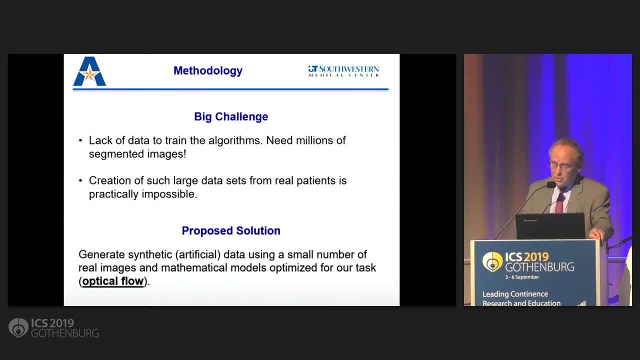 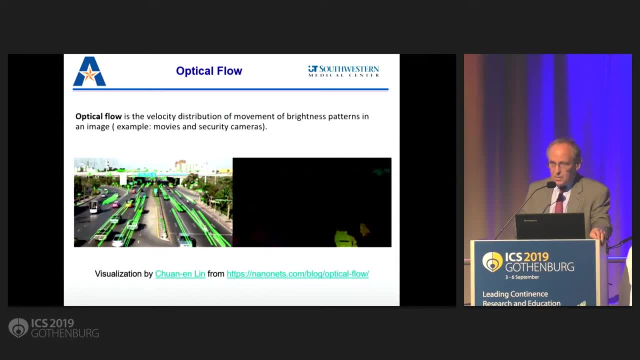 of patients that we can import into our data set. So the purpose solution is here. what they're proposing is called optical flow, where you can see the same images progressively over time and with modeling you can predict where the object will be in the next fraction. 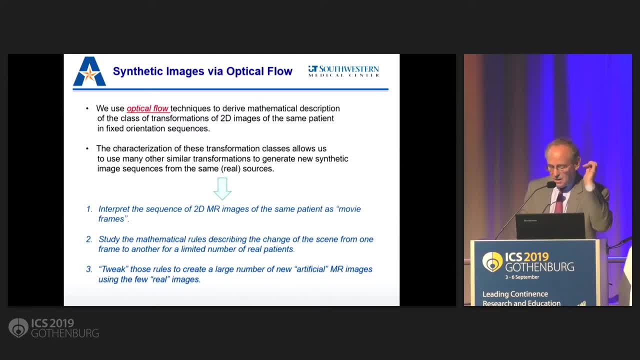 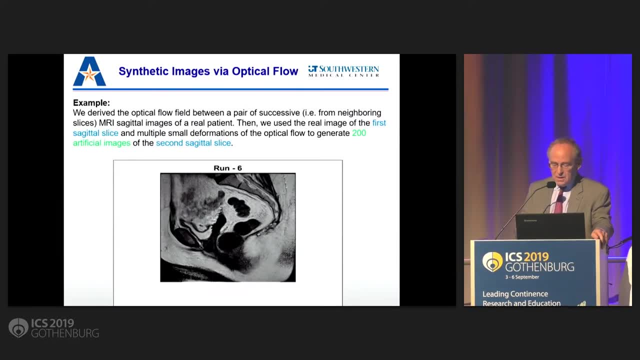 of seconds. So they take basically two images and then they create lots of artificial images in between. So, for example, here you'll see, between the slice, One is on the top of the image and the other is at the bottom, And this is to do with the analyzing of the pictures. 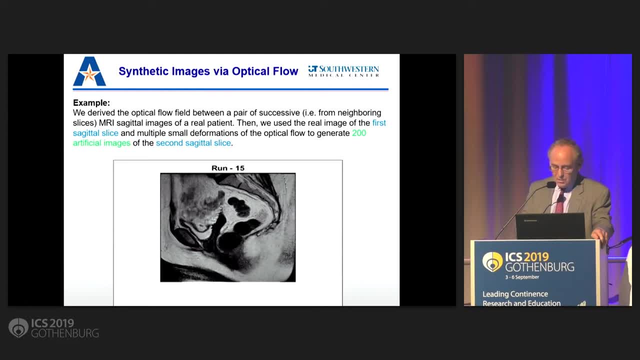 so, in order to be able to do this, you have to start from the very beginning, And then we have to pick up any of the images and try to consider which object might be available, which satchel view in size 200,- and I won't run to 200, but with a little tweaking of the 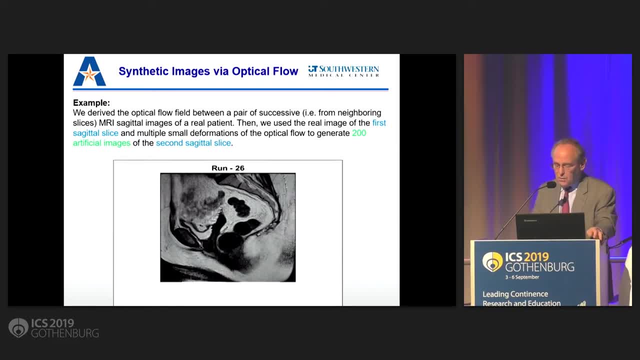 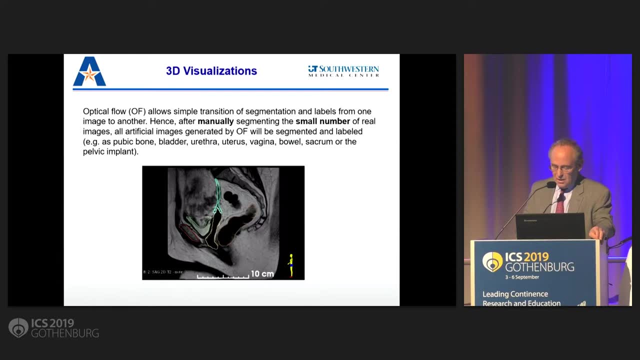 model. they can create some artificial images between the first and the second slice and they can then import that into the model. So if you then manually segment that, you can determine in the front of these images where the pubic bone is, the bladder, the vagina, the rectum, and then you can figure. 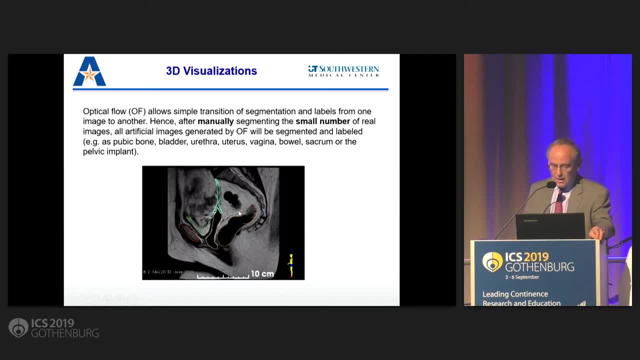 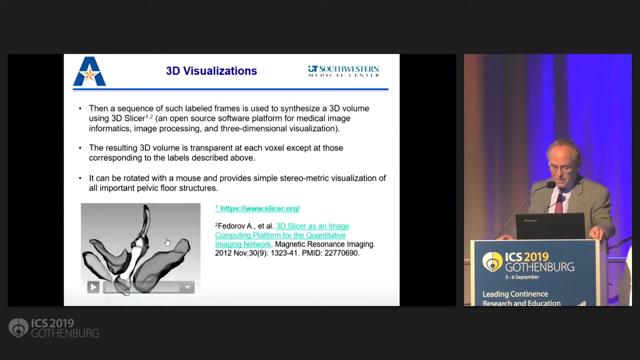 out where that mesh, that mesh ecoclopopex is located pretty accurately, And so they then bring this into 3D slicers and they can then make this beautiful rendering that they have here. So that part of the technology is straightforward. 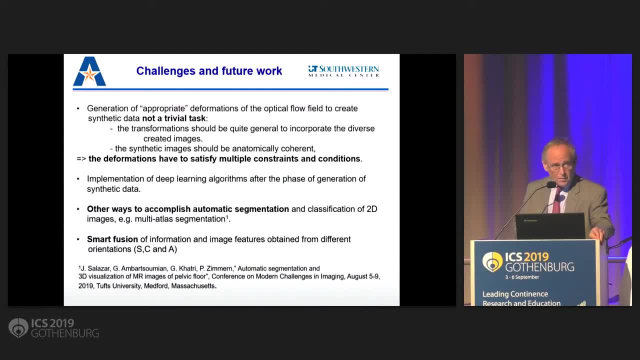 So there are challenges because, even though I tried to simplify it, for you and for me as a urologist not having any expertise in mathematical modeling, it's not a trivial task. The transformation process is complicated and they have to satisfy multiple constraints. 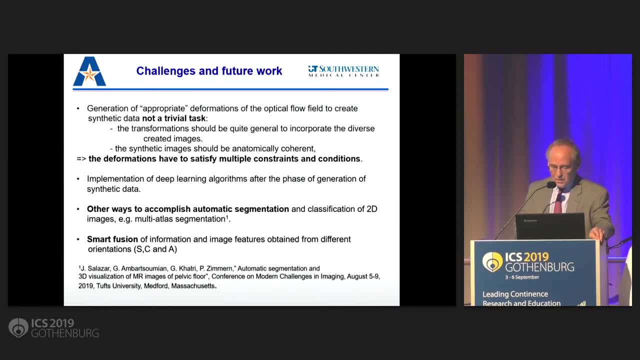 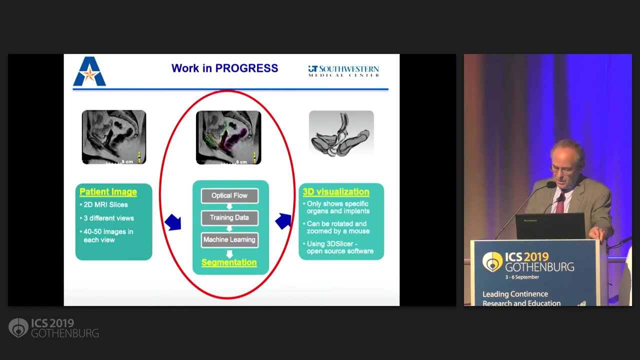 and conditions, And they're also exploring other ways of doing this with smart fusion And multi-atlas segmentation, which are other techniques that they are using in their fields for image analysis. So here is basically the summary of the work in progress. So far we've worked about 10 patients. 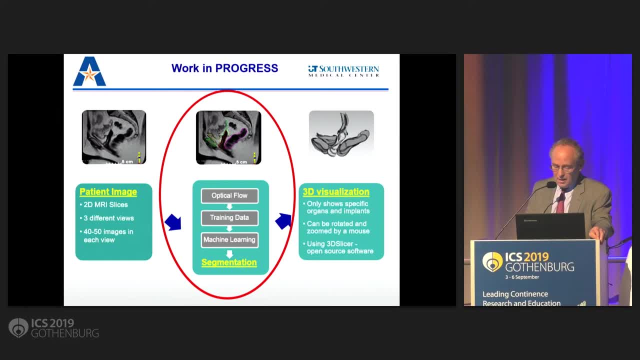 We have recently gone to 20, and we're working to an NIH grant submission at present. Thank you, Questions please. Well, as a surgical gynecologist, I find your technique seems very, very valuable. With time, do you think you will achieve the speed to have dynamic pictures? 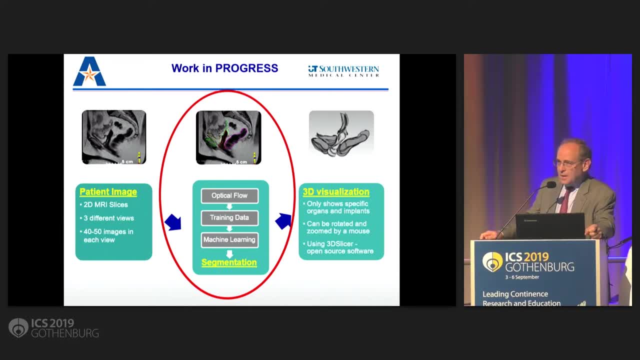 This is static, as I understand you. Yeah, it is static right now, but they can create as many images as they want. Basically, it's the mathematical formulation between slices that is the tricky thing. So when you can basically create a flow, like you know, it's basically doing from images. 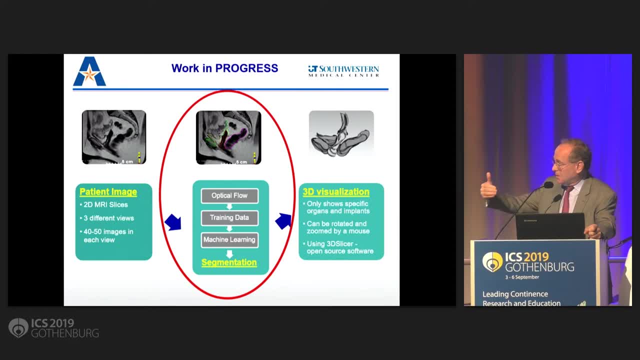 to movies. So you see something flowing. they can do the same with the technology. So you see an image, I see an image. they move to the next image and in between they create a bunch of images which are extremely different but very. you know, you can't pick. 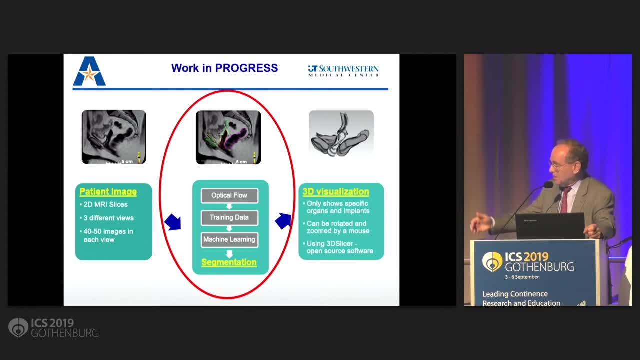 up the difference, but they can, And they can basically make that a dynamic process. yes, Very interesting, So you think, because I think that it's not only for taking out some mesh, it could also be: how does meshes change the physiology of the area?